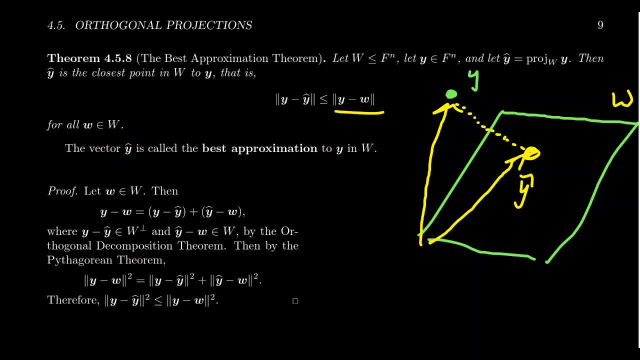 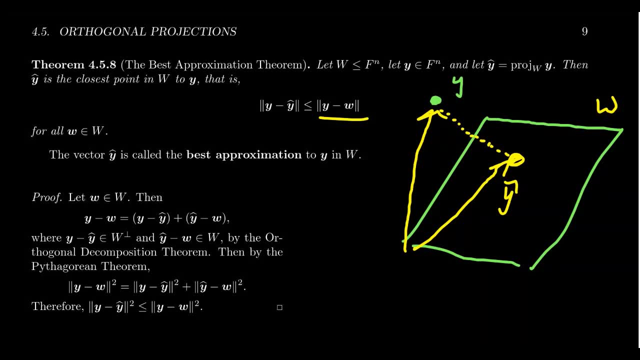 closest vector in w to y, And the proof is pretty slick: It's a, very, it's a. it's a quick application of the orthogonal decomposition theorem we saw in the previous video. So take any vector little w inside of w. Well then we're going to take a look at the difference. 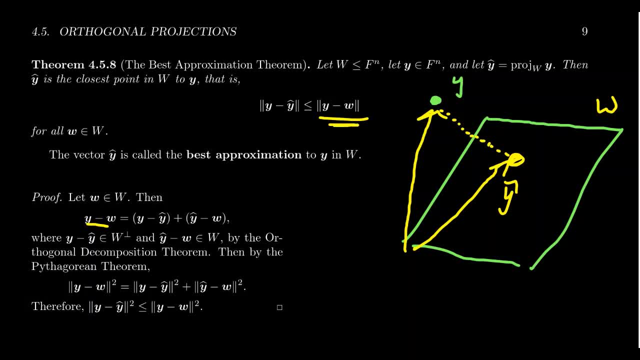 between y and w. We want to show that the length of this vector is bigger than y minus y hat, the orthogonal projection of y into w. Well, first of all, we're just going to insert y hat into the equation, right? So take y minus y hat plus y hat minus w, right there, Notice, of course. 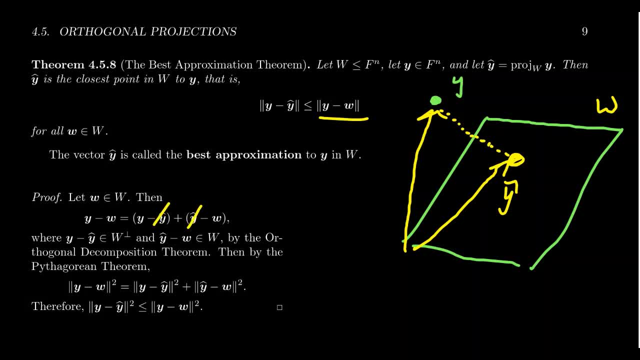 y hat minus y hat. they can't size get back a y minus hat here, excuse me, a y minus w right there. Why is this sum important? This is actually the orthogonal decomposition that's guaranteed by the orthogonal decomposition theorem, right? So notice that y hat belongs to w the orthogonal projection. 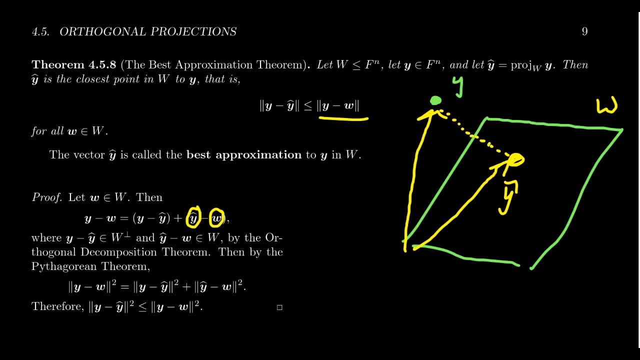 does, And w is just some arbitrary element inside of big W, And so the difference is a linear combination of vectors in w. Since it's a subspace, it'll be in there, So this vector belongs to w. On the other hand, we've already seen previously that y minus its orthogonal projection onto w. 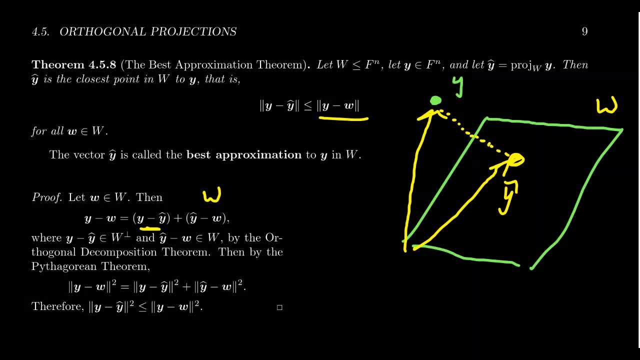 is itself orthogonal. It's orthogonal to vectors in w. This is something that belongs to w perp, as we've seen. So this is the orthogonal decomposition of y minus w. In particular, these vectors are perpendicular with each other. This is relevant because of the Pythagorean equation. 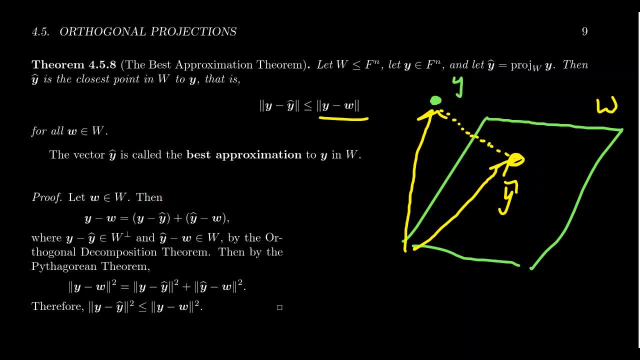 If we have a sum like this, if we have this orthogonal decomposition, we know that if we take the norm of y minus w squared, this is going to equal the norm of y minus y hat squared plus the orthogonal decomposition of y minus w squared. 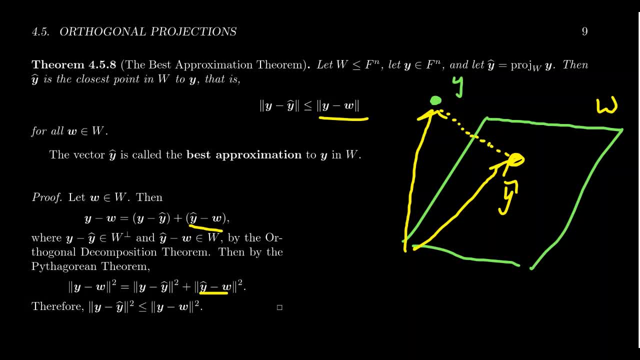 The norm of y hat minus w squared like: so Now these are all non-negative quantities because our norm satisfies this positive, definite condition. If I were to remove some positive side, some positive quantity on the right-hand side, that makes the right-hand side get smaller And 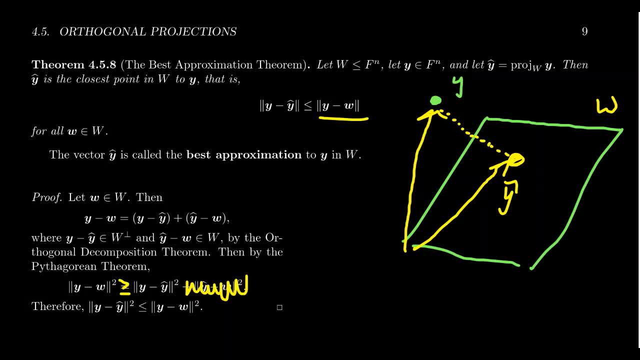 so we no longer have equality, We have an inequality. Y minus w length squared is greater than equal to the length of y minus hat squared. Taking the square root, we've then established the inequality given to us by the vector, So we have an inequality of y minus w squared. 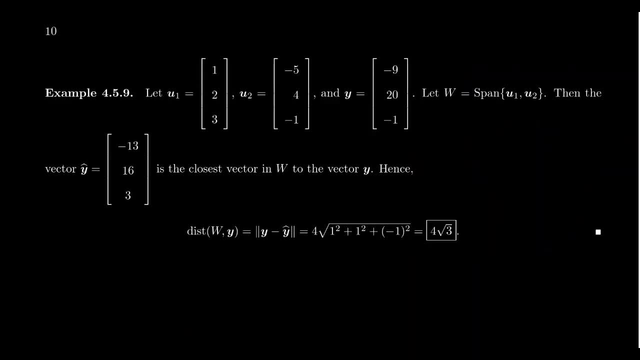 This is the best approximation theorem. Let's see an example of such a thing. Let's take two vectors, u1 and u2, 1, 2, 3, and negative 5, 4, negative 1. This will be a spanning set for w, but this is also, in fact, an orthogonal. 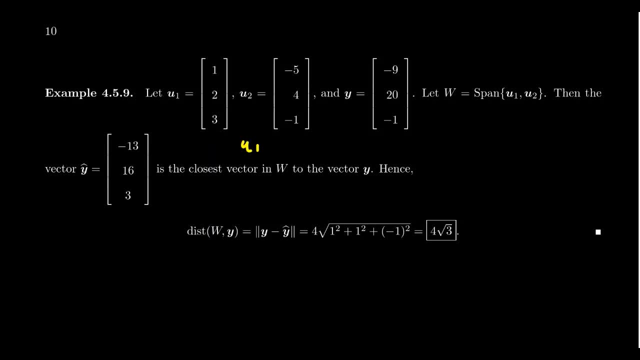 spanning set an orthogonal basis for w. Notice, if I take u1, dot u2,, you end up with negative 5 plus 8 minus 3.. That gives us a zero right there, And so then we showed in a previous video. 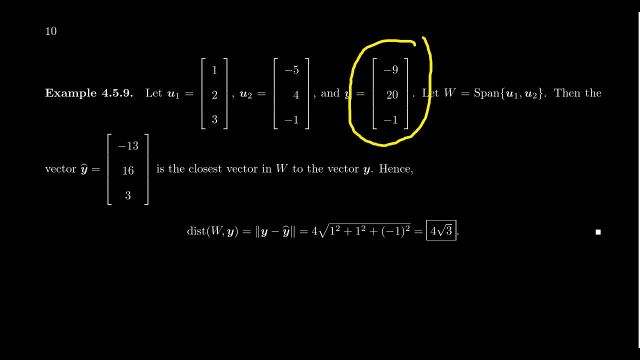 that if you take the vector y, that its orthogonal projection onto w is going to be this vector right here, negative 13,, 16, and 3.. Therefore, the distance between y and the space, the plane, w is going to be the distance between the plane and the vector, is going to be the distance between y. 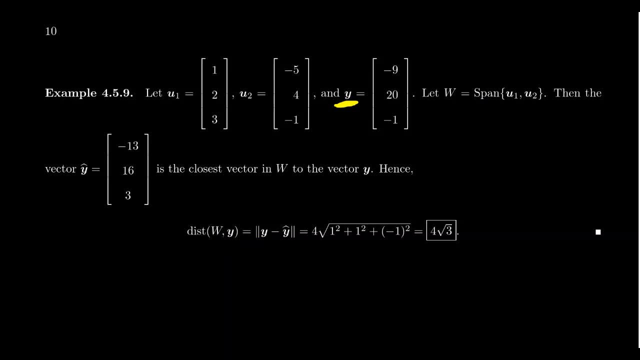 and its orthogonal projection, For which, if we calculate the difference of this thing, we're going to take negative 9 minus 13.. Here we get y minus y half. This is going to equal a 4.. If we take 20 minus 16, that's also. 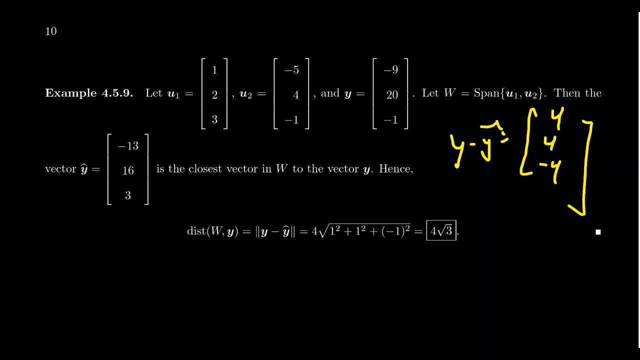 4. If we take negative 1 minus 3, that's a negative 4, like. so You can factor out the 4 out, so you get 1, 1, and negative 1.. And so then the length of this thing is going to be 4 times the square. 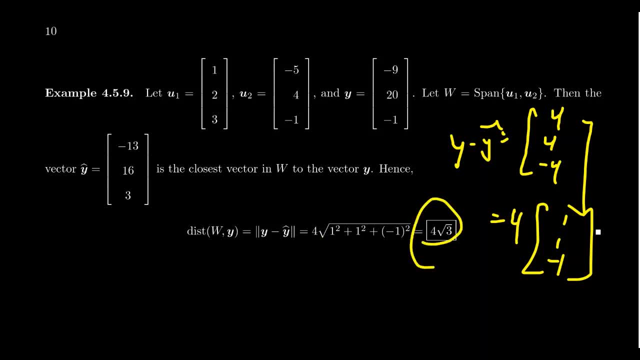 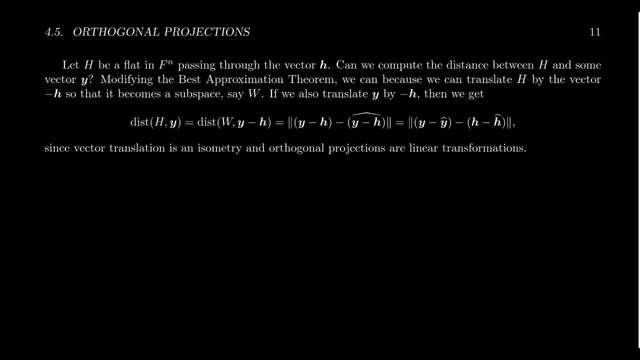 root of 1, 1, 1.. That is, we get the distance of 4 times the square root of 3.. So we talked about the distance we can find between a vector and a subspace, but can we do that for any affine set? 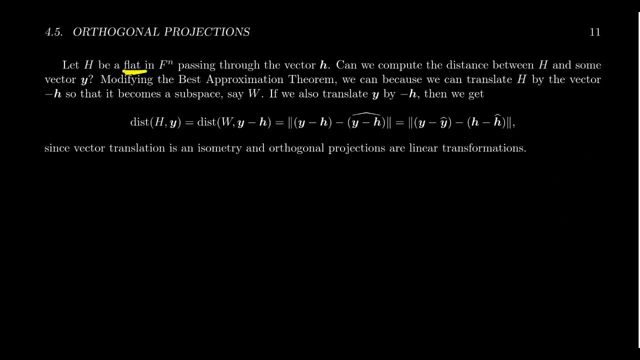 for any flat. Well, up to translation, every flat is just a vector space. So what we could do is, if we have, if we have some flat capital H and it contains a particular vector, little h, we could just subtract little h from it so that h then becomes a subspace. It'll then be a subspace that passes. 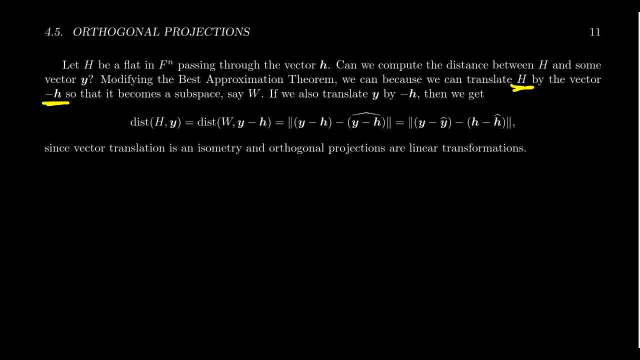 through the origin. Let's now call it w, And so if we want to calculate the distance, so if we're looking for the distance between h and y, this is the same thing as the distance between w and y minus h. So we just translated the flat into a flat through the origin, aka a subspace, And then